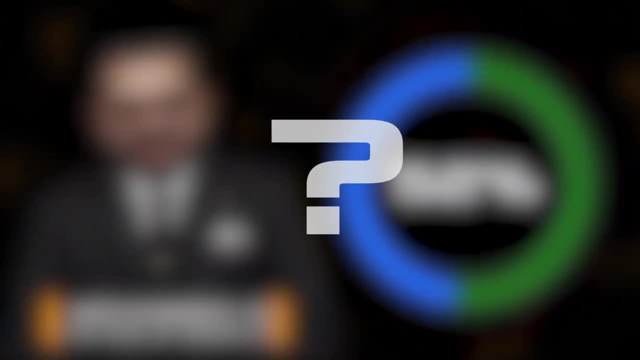 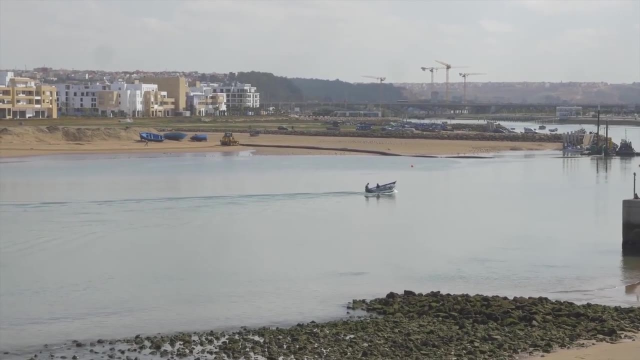 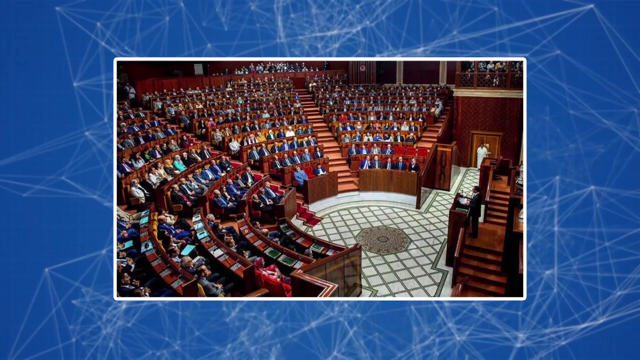 using green energy by 2030. But how will it be achieved? Hydro resources in Morocco are bad. most of the rivers dry up and reservoirs built in the 1960s provide the population with drinking water, but their energy source is limited. In 2008,, the authorities adopted the New Energy Strategy. 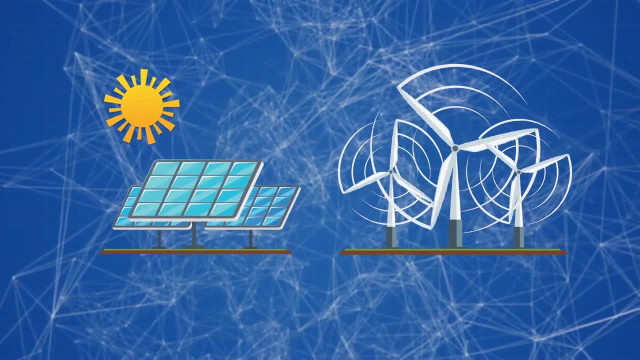 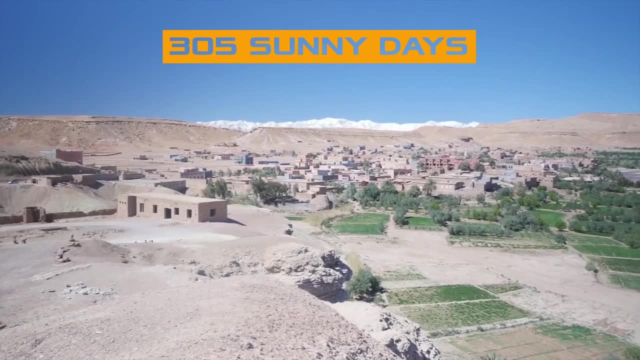 Energy. According to it, the sun and wind are the most important types of energy to use. It is logical for a country where the number of sunny days per year is over 300.. As part of the strategy, the Office of Energy Efficiency and Renewable Energy, the Moroccan. 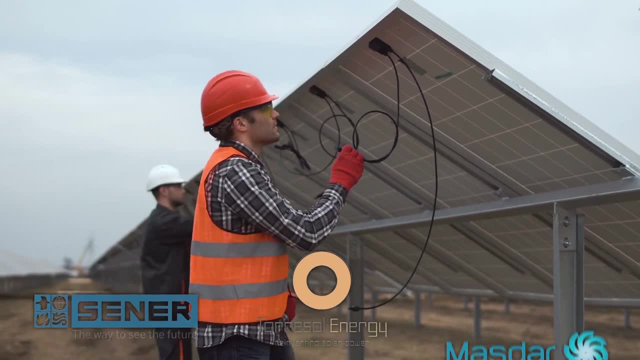 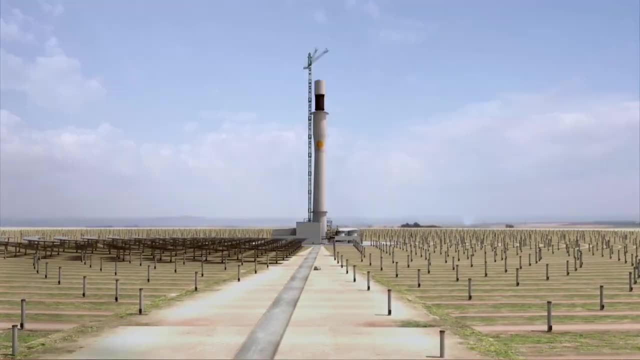 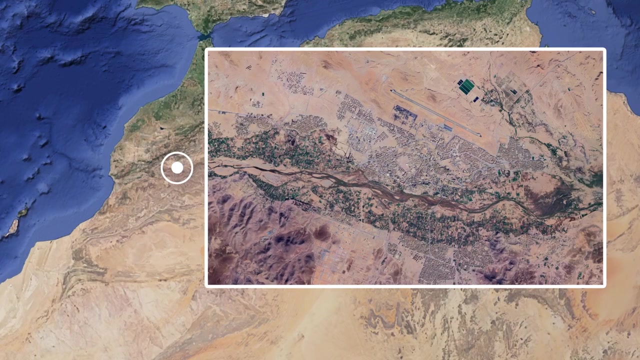 Agency for Solar Energy, as well as several research organizations and investment funds specializing in green energy, were created. The Noor Ur-Zazate solar power plant was the first solar project developed under Morocco's new energy strategy. Ur-Zazate is a city located in the Moroccan desert. 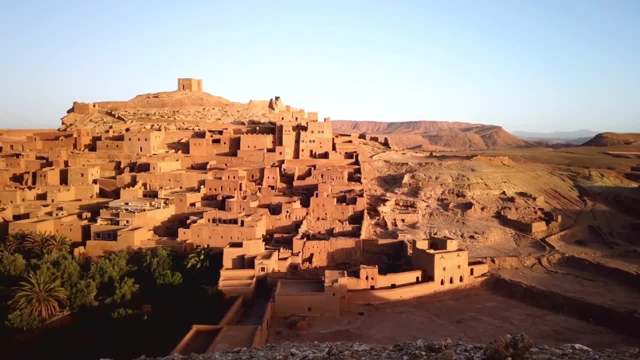 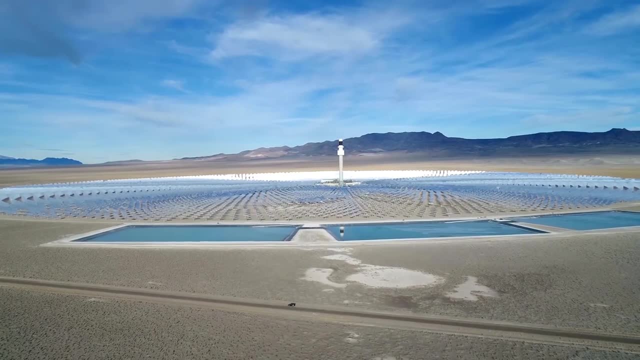 It's famous because popular films, as well as TV shows, were filmed here: Lawrence of Arabia, The Mummy, Game of Thrones. But now the name of the city is associated not with the cinema, but with the world's largest Ur-Zazate Concentrated Solar Power Station. 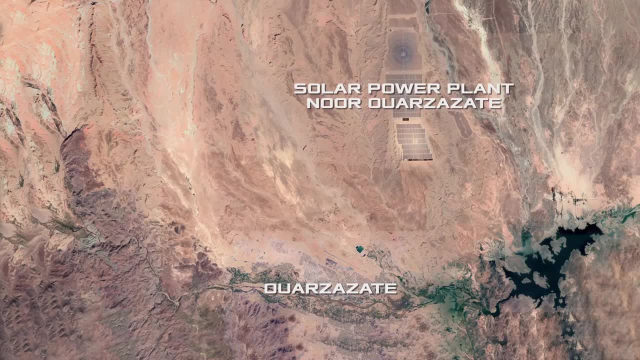 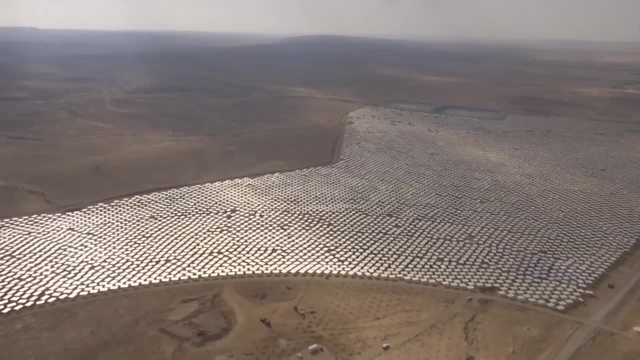 It is located in the Atlas Mountains in the western part of the Sahara, 20 km from the provincial capital of Sammasa-Dra Ur-Zazate. This location was chosen because the level of annual solar radiation here is 2,635 kilowatt-hours. 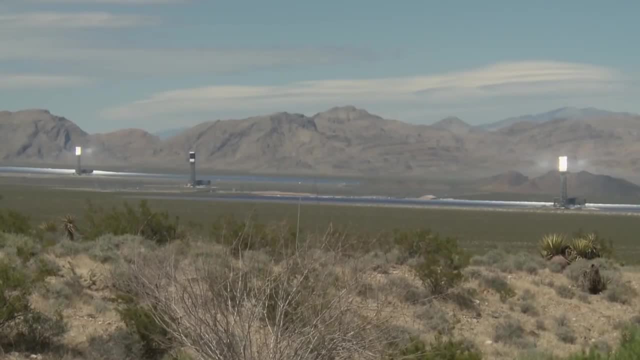 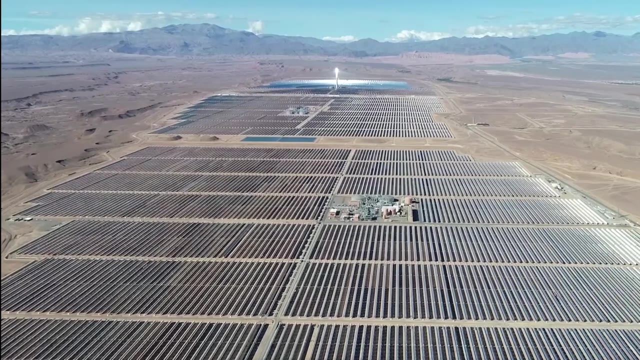 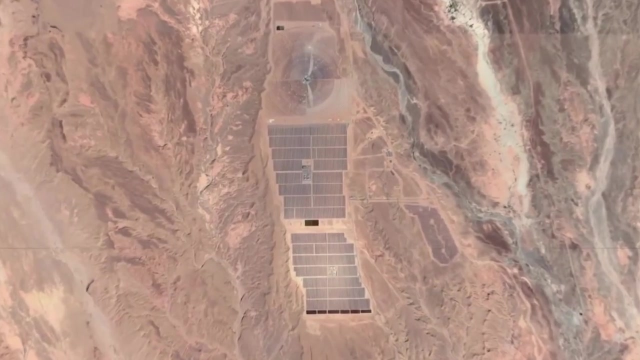 per square meter. This is one of the highest rates in the world. The sun shines here, with rare exceptions, 365 days a year, Spread out over 3,000 hectares, the equivalent of 3,500 football fields. the solar complex consists of four separate solar power plants, each using different technologies. 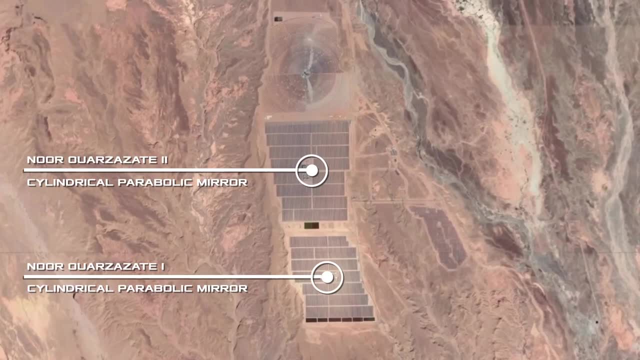 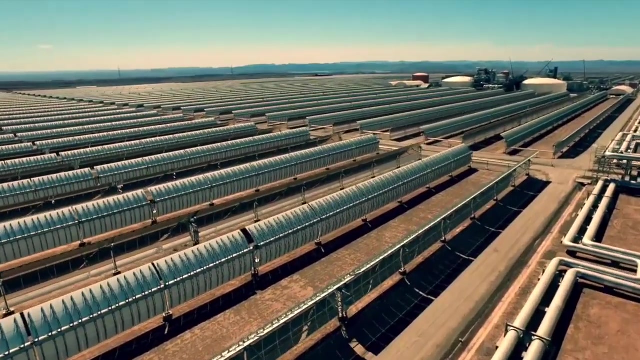 Nur Ur-Zazate 1 and 2, Cylindrical Parabolic Mirror. Nur Ur-Zazate 3, Solar Power Tower. Nur Ur-Zazate 4, Photovoltaic Plant. The construction of the first section began in 2013 and work on the last section was completed. 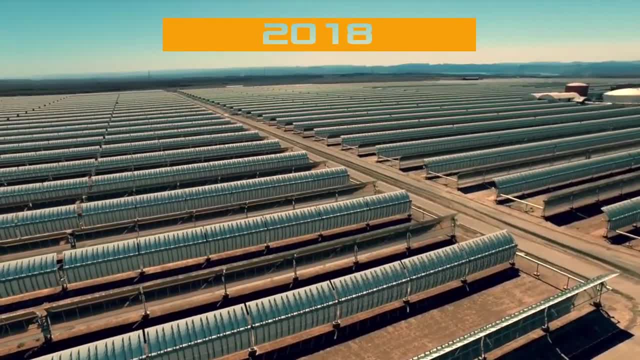 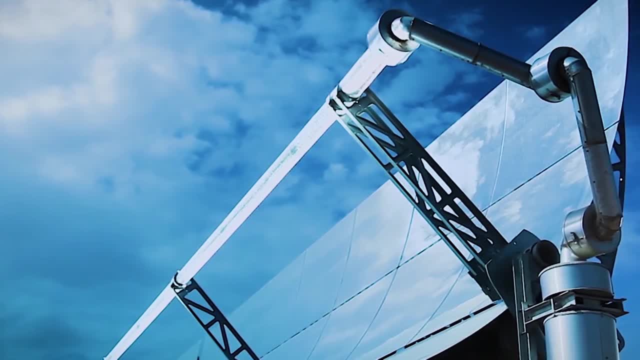 in 2018.. The power plant is based on the technology of concentrated solar energy. The system uses a large array of mirrors or heliostats to concentrate the sun's rays. These beams heat a fluid that creates steam to drive a turbine and generate electricity. 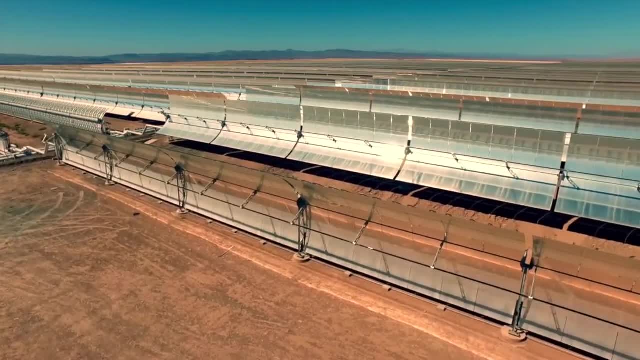 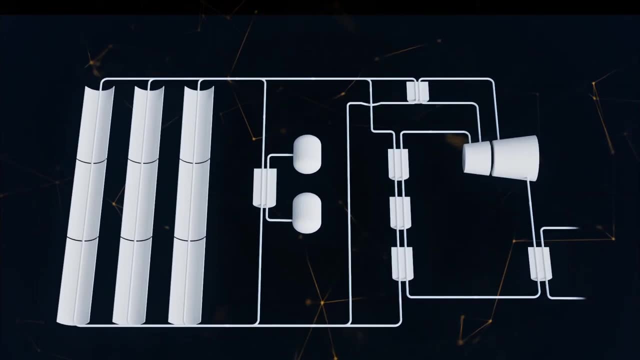 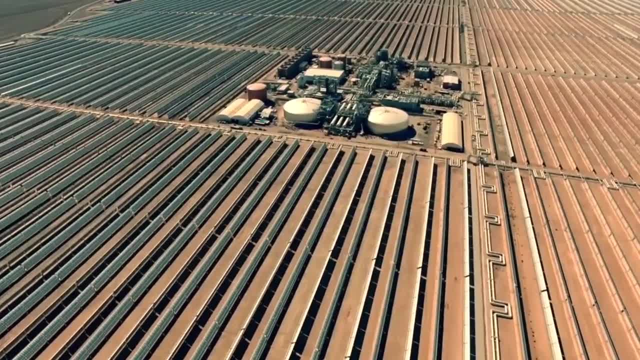 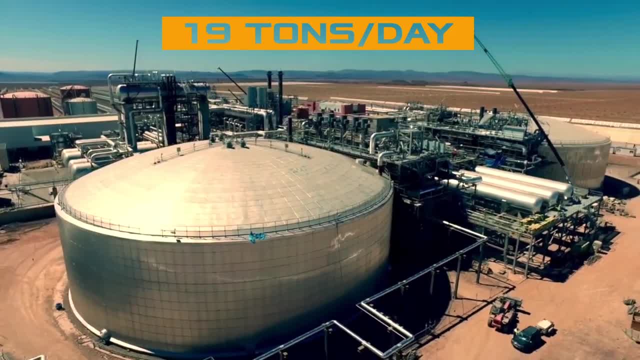 The solar power plant is used to generate electricity. It is located low, above 110°C, and the temperature of the synthetic oil of the heat carrier is above 8°C. Nineteen tonnes of diesel fuel are needed per day. However, each section of the power plant has its characteristics of functioning. 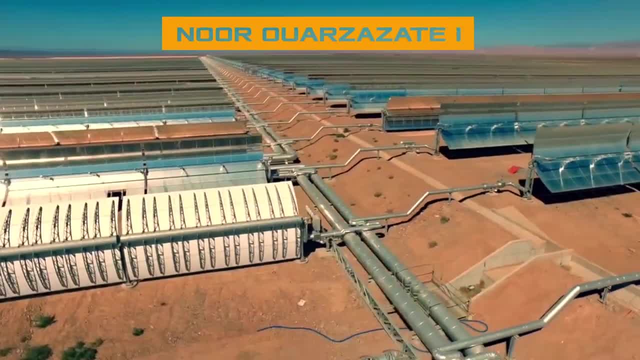 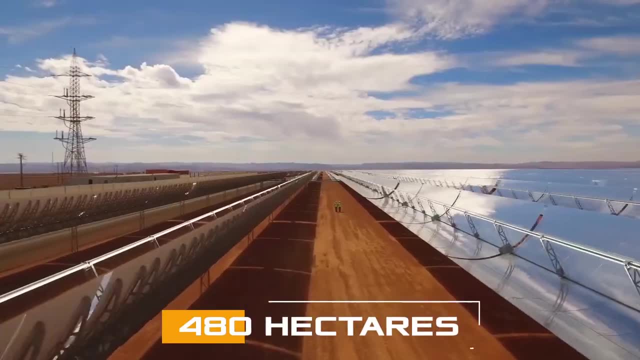 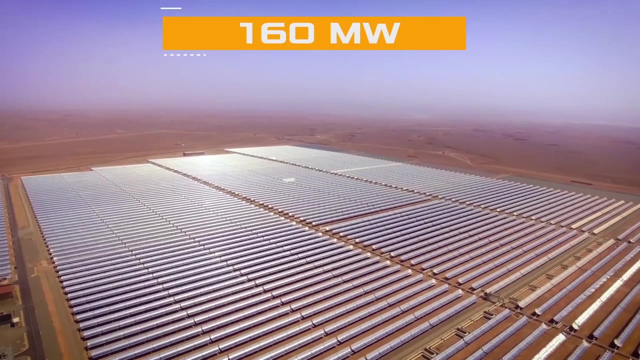 The first phase of the complex Nur Ur-Zazate I was inaugurated by King Mohammed VI in 2016.. The first stage of the solar power plant includes 480 hectares of centers center trough cylindrical parabolic mirrors. The installed capacity is 160 megawatt. 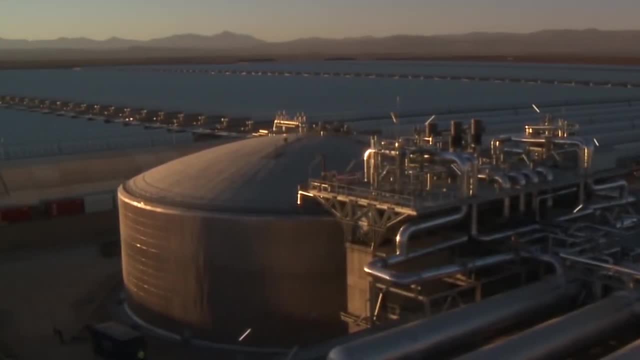 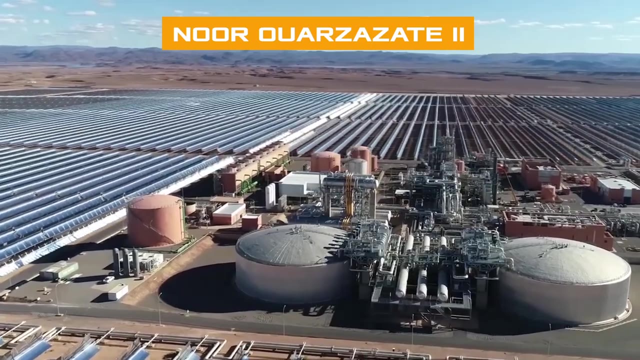 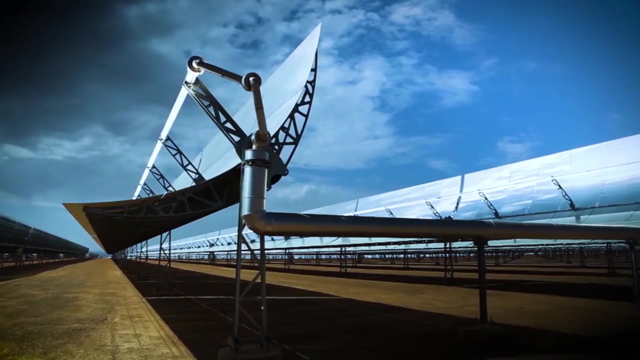 The facility provides storage of electrical energy in a salt reservoir for three hours. The second phase of Uruzazate covers an area of 600 hectares. Its installed capacity is 200 megawatt. It uses solar energy concentration with dry, air-cooled parabolic mirrors without water. 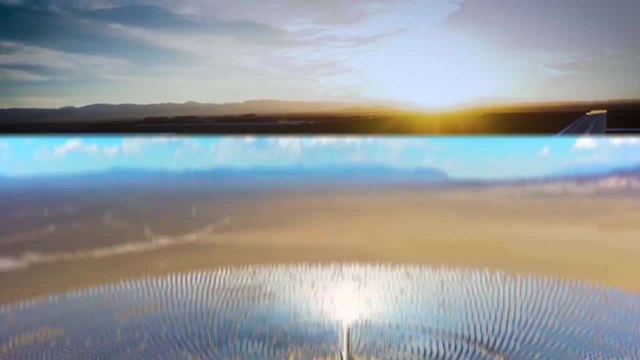 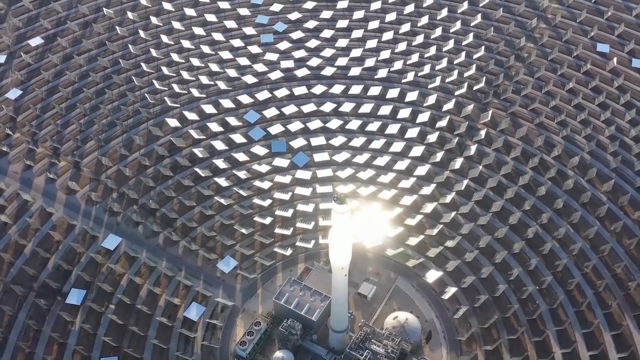 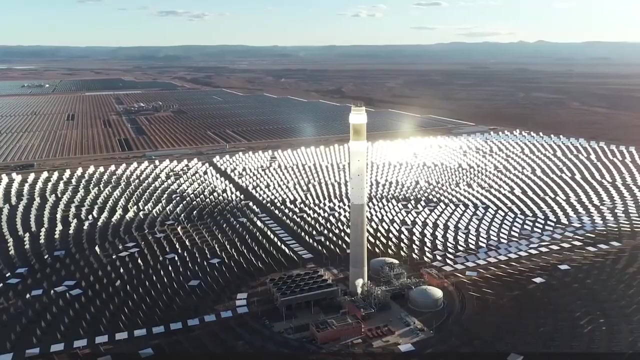 The system saves electricity for 7 to 8 hours. Nor Uruzazate 3,, put into operation in 2018, was the first power plant in Morocco to use dry-cooling solar tower technology. Instead of rows of mirrors, this line collects solar energy with the help of one large tower. 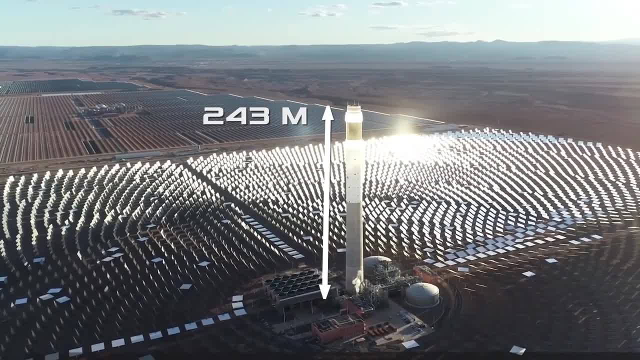 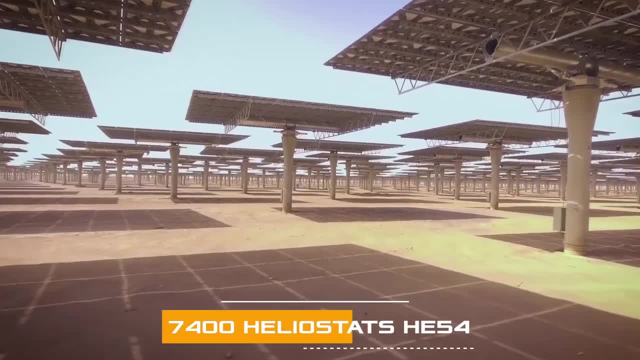 243 meters high, pluralistically the highest in Africa. In this way, significant space savings can be achieved. The system uses 7,400 centers, HE54 heliostats or mirrors, each with an efficiency of up to 1,000. 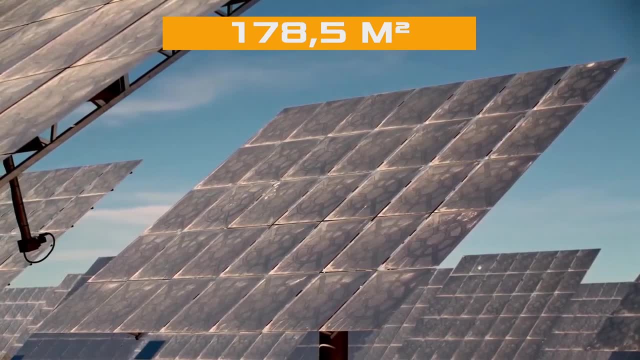 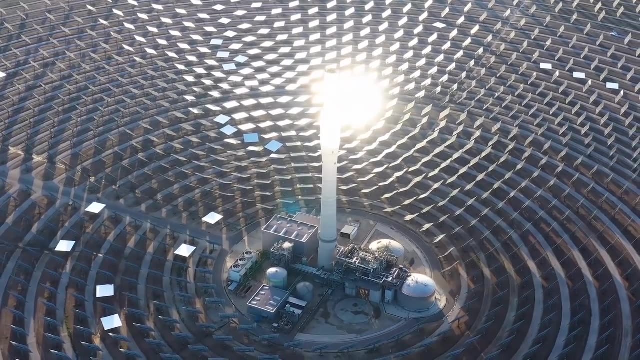 The system has an effective area of 178.5 square meters and equipped with a high-precision hydraulically-driven solar tracking system. The mirrors turn to follow the sun and direct its light to a tower receiver mounted on the top of the structure. 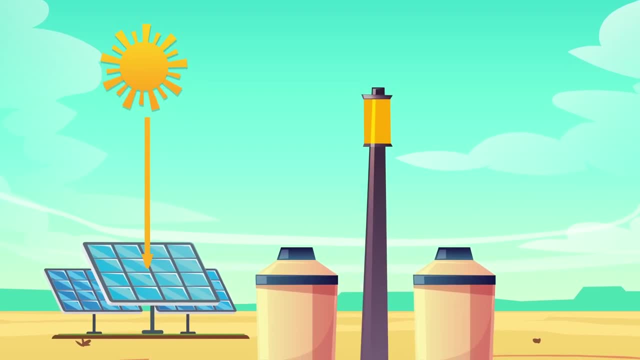 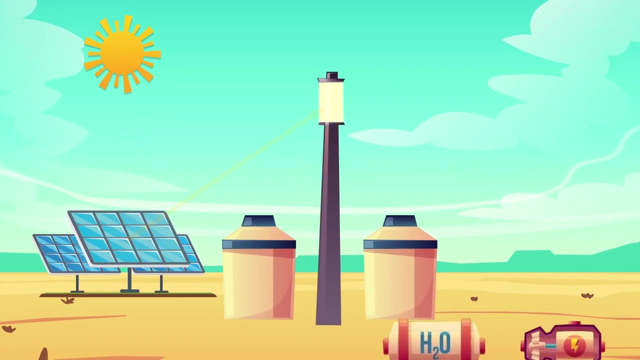 The tower is filled with a salt mixture which is heated by the sun's rays to 565 degrees Celsius. This is higher than when using mirror fields, so the station does not require the use of fuel to maintain the temperature of the salt mixture. The hot air is used to heat the tower. 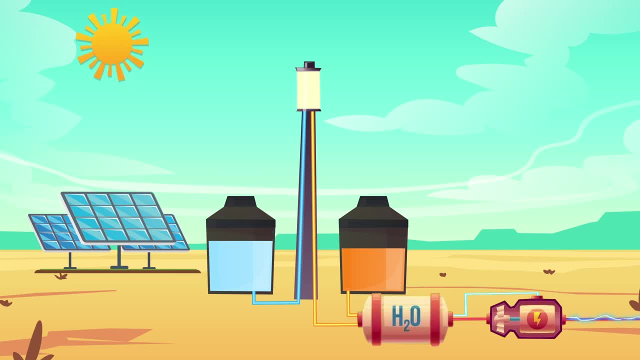 The hot salt drains into a stainless steel tank after passing through a heat exchanger to heat water and generate steam to power a turbo generator. The capacity of the tank allows accumulating enough molten salt to guarantee the supply of electricity up to 7 hours after sunset. 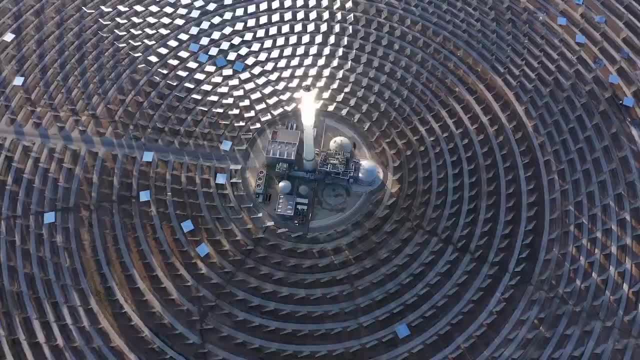 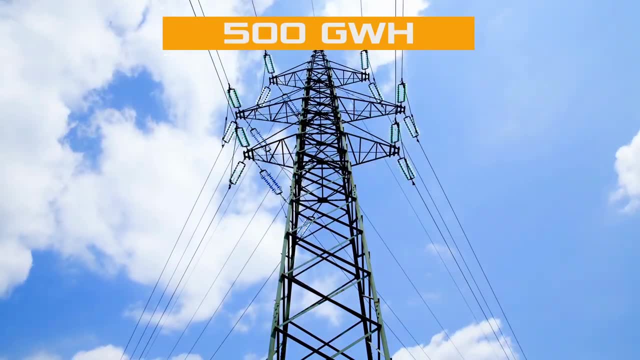 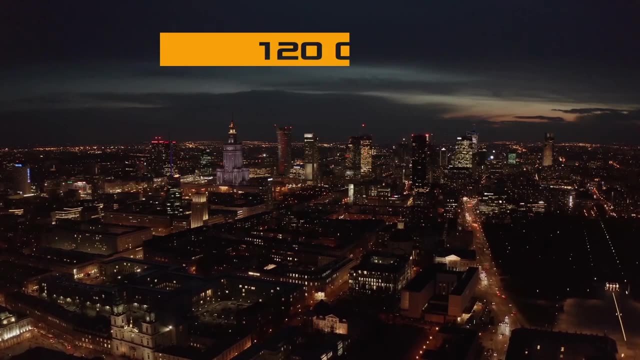 The facility covers an area of 582 hectares and its installed capacity is 150 megawatt. Annual electricity generation is 500 gigawatt hours. The price of energy produced is 14 cents per kilowatt hour. Once operational, the station generates enough green energy to power 120,000 homes. 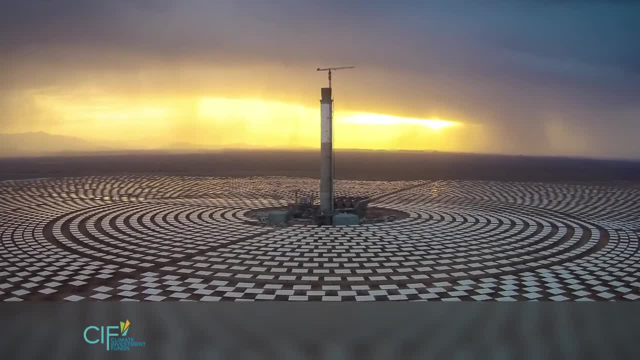 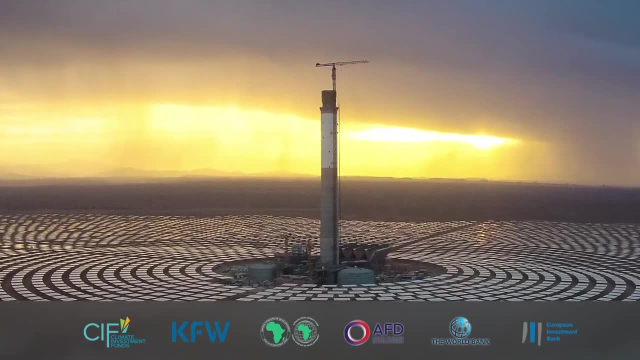 Nour Orazazate III's investors are the Clean Technology Fund, KfW, the African Development Bank, the French Development Agency, the World Bank and the European Investment Bank. The cost of the project is about $700,000. 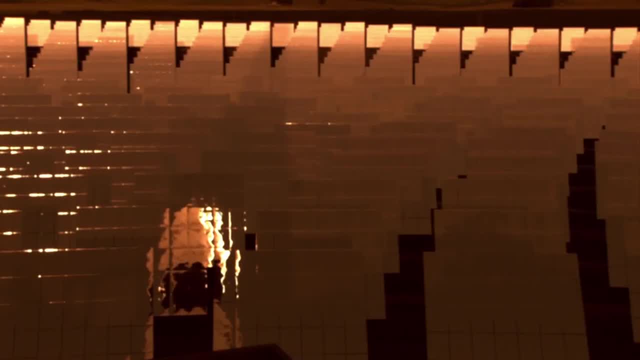 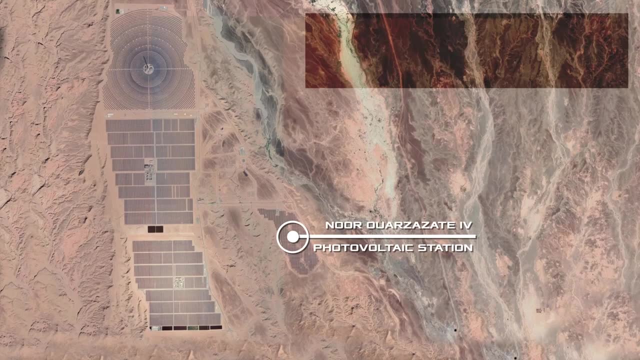 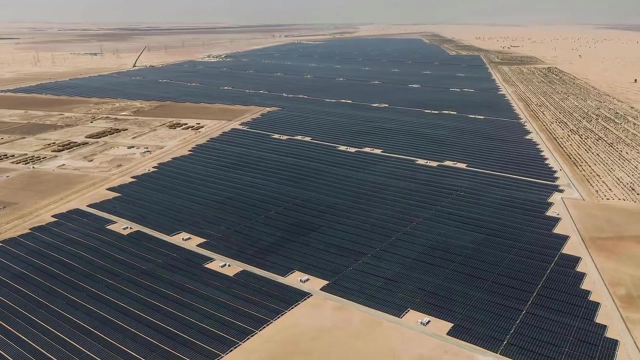 A solar power plant that produces electricity Even at night. What could be more amazing? Note that the fourth and last station of the solar power plant complex with a capacity of 72 megawatt and an area of 137 hectares that has an installed capacity of 72 megawatt. 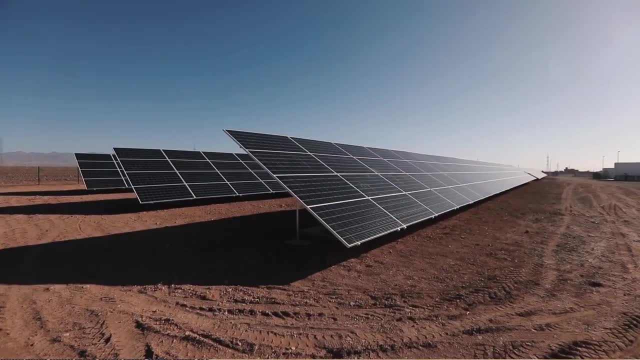 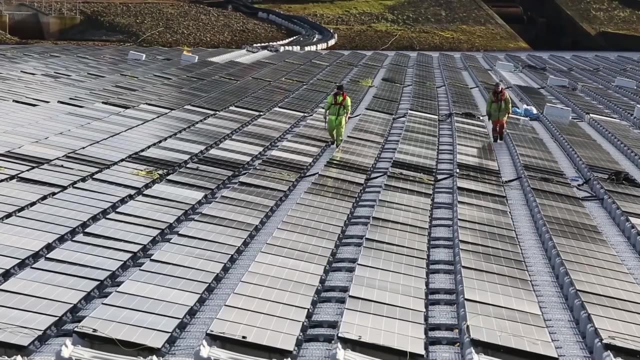 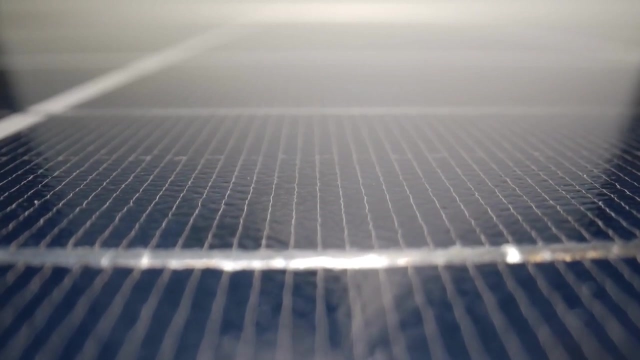 is also a technological novelty Here. for the first time, hybrid photovoltaic technology has been applied, which combines traditional photovoltaic cells used on solar panels that are familiar to us with concentrated solar energy systems, which are used at three other Nour Orazazate stations.